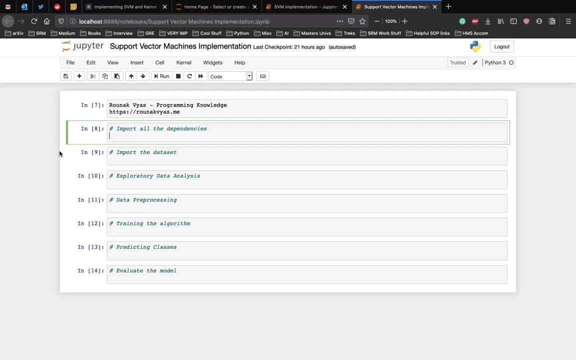 We'll talk about implementing support vector machines. My name is Ronak Vyas and this video is a collaboration with Programming Knowledge. To watch more videos on machine learning and programming, do subscribe to the channel. A support vector machine is a type of supervised machine learning classification algorithm. SVMs were introduced initially in the 1960s. 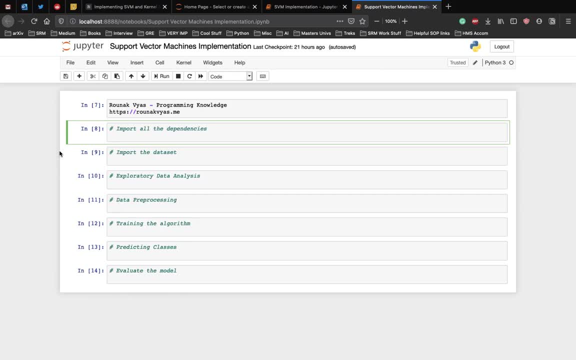 and were later refined in 1990s. However, it is only now that they are becoming extremely popular, owing to their ability to achieve brilliant results. SVMs are implemented in a unique way when compared to other machine learning algorithms. In this video, we'll 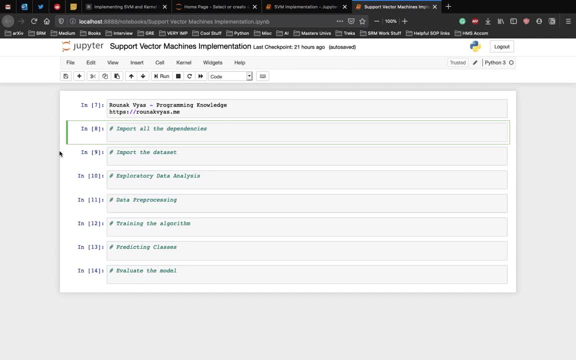 implement support vector machines with the help of the scikit-learn library For the implementation. our task is to predict whether a bank currency note is authentic or not, based on four attributes of the note. Those attributes are: the skewness of the wavelet performed. 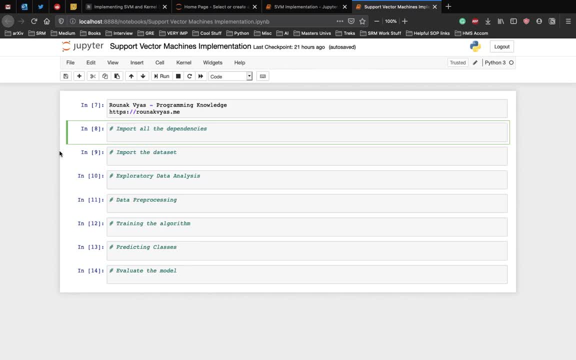 image, The variance of the image, Entropy of the image and the kurtosis of the image. This is a binary classification problem and we will use the SVM algorithm to solve this problem. The detailed information about the data and a link to download the dataset can be found. 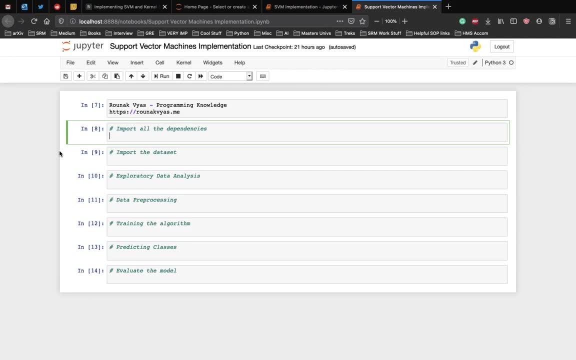 in the description: Download the dataset and store it locally on a computer where you intend to write the implementation. So let's start the implementation by importing all the necessary libraries. First, we need to import pandas, as we need to store our data in a data frame. 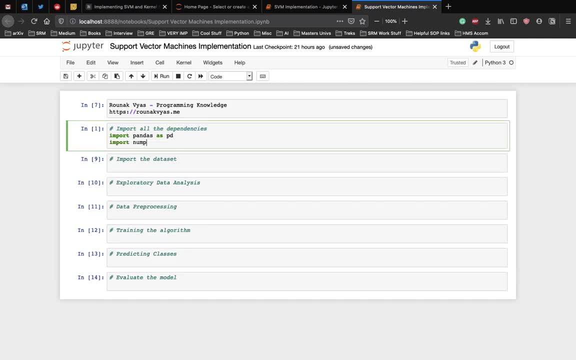 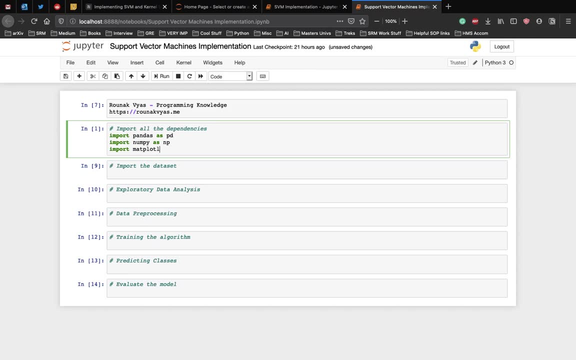 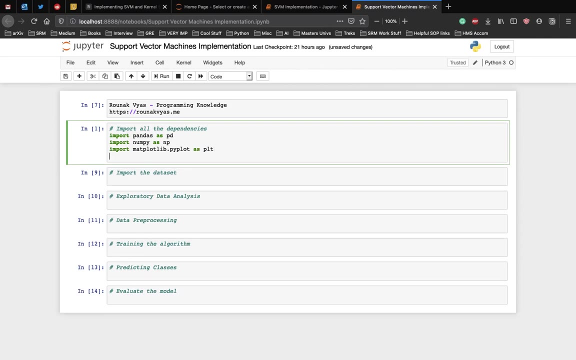 And the next is numpy, Followed by matplotlib, And then we need the scikit-learn modules, And then we need the scikit-learn modules, And then we need the scikit-learn modules. Its gonna be hard to find any module same as a ماal in a byte can be, and such. 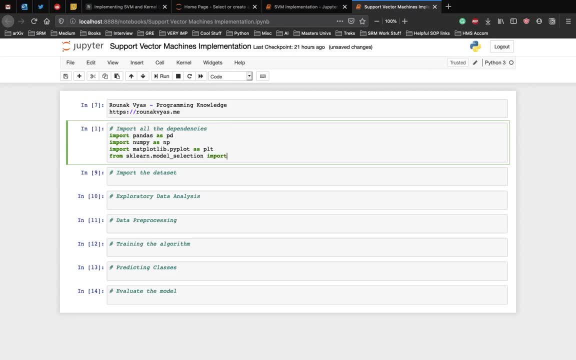 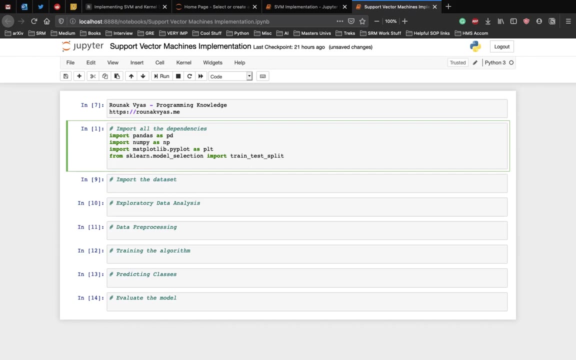 So we will leave it aside, but we will cut this Thermal enormously And let's go for 구입. Here we will be using the train test split module which we have had, not in the previous video for linear & logistic regression implementations, But for SVM. we'll actually have a train test split and see how the algorithm works on the. 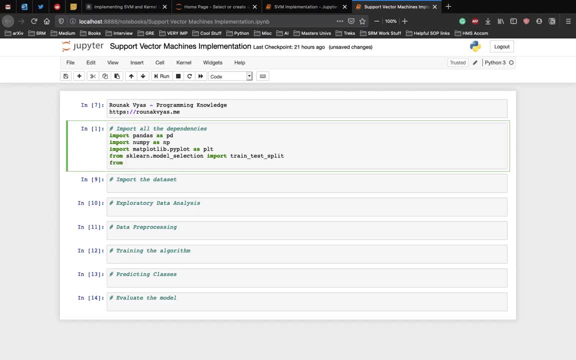 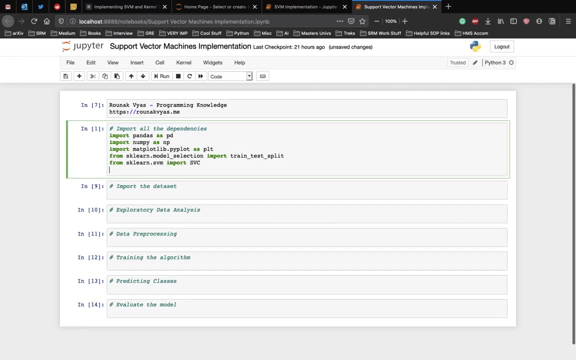 test data. Next, we need to import the SVM class, which is SVC support vector classifier, and at last, we need to evaluate our algorithm. so we'll need some metrics for that and let's use the classification report module and, yeah, I think we're done. 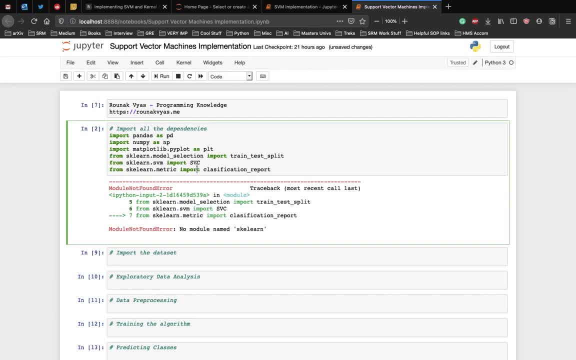 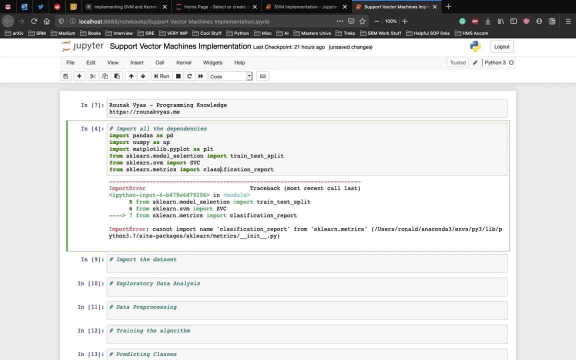 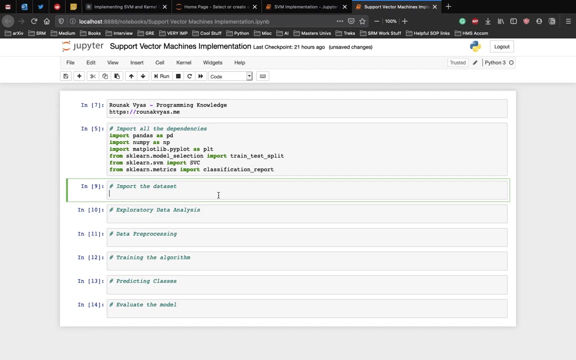 So now let's import the data. okay, I think we have some problem. yeah, it's a spelling mistake. metrics have a lot of spelling mistakes here. okay, Now let's import the data into our program. To read the data from the CSV file, the simplest way is to use the read CSV method of the Pandas. 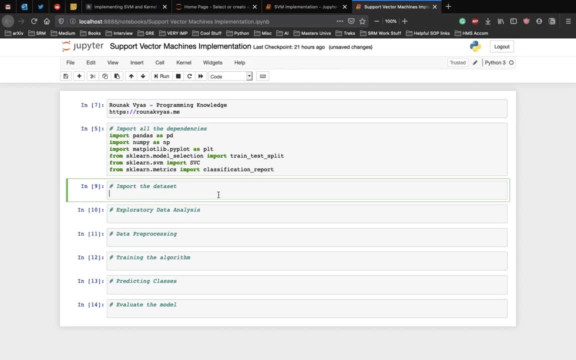 library. The following code which I'm going to write is going to read the bank currency node data into a Pandas data frame. Let's have bank data equal to PD dot read CSV, and the name of the CSV file is bill authentication, which you can find in the description of the video. 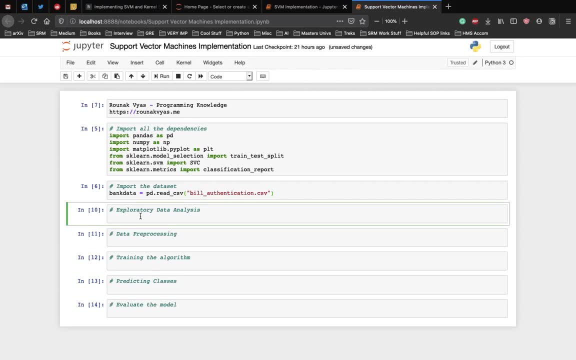 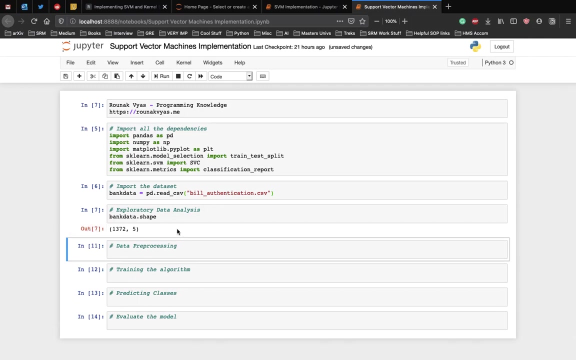 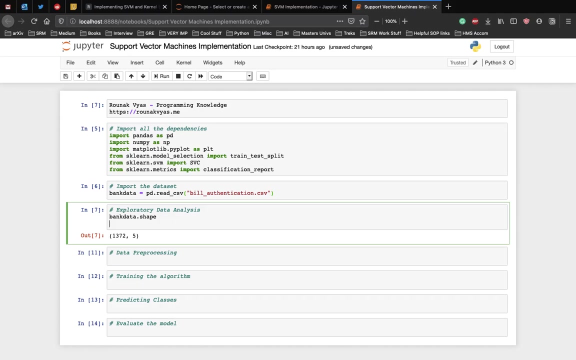 Okay. now they are virtually limitless ways to analyze data sets: user rows, clouds という data set. Okay set has 1372 rows and 5 columns. Now to get a feel of how our data set actually looks, lets actually see the first 5 rows of the data set using the head command And here: 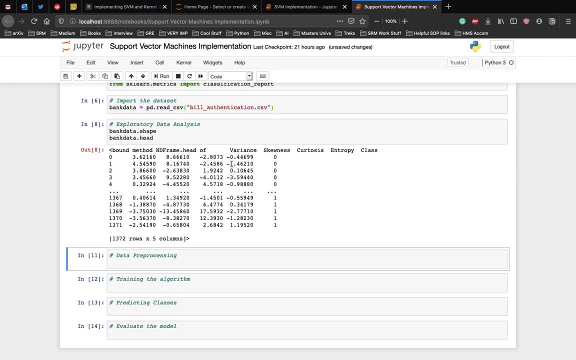 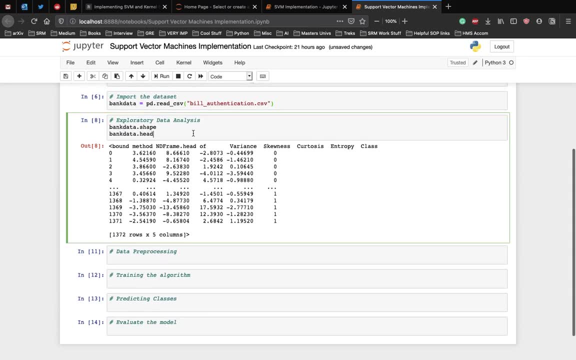 you can see the first 5 rows of data set and you can also see the attributes of the data set are numeric. The label is also numeric, that is class 1 or 0.. Lets preprocess the data before training the model. Data preprocessing involves two steps. First, dividing the data. 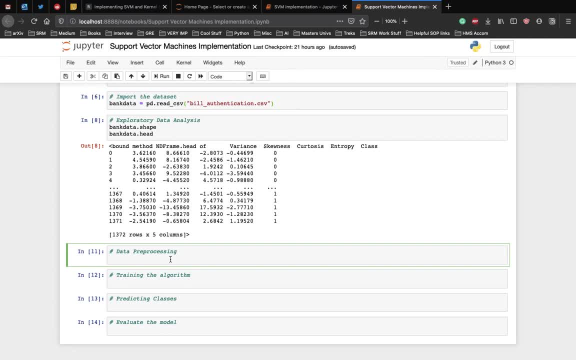 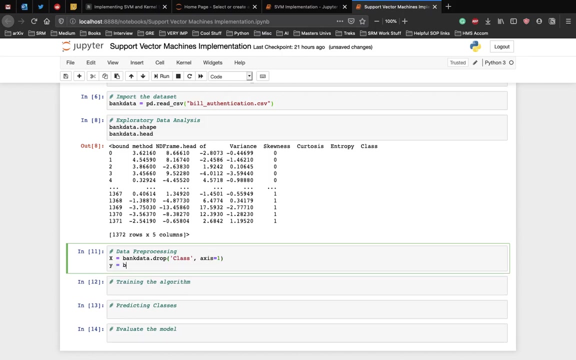 into attributes and labels and second, dividing the data into training and testing sets. To divide the data into attributes and labels, execute the following code: Let x equal to the attributes, So bank data, dot drop 1 and y equal to bank data class, which is the label In the first. 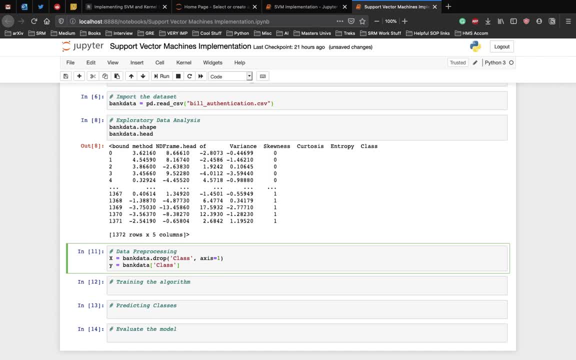 line of the script in the cell. all the columns of the bank data data frame are being stored in x, except the class column, which is the label column. The drop method drops this column. In the second line, only the class column is being stored in the y variable At this point. 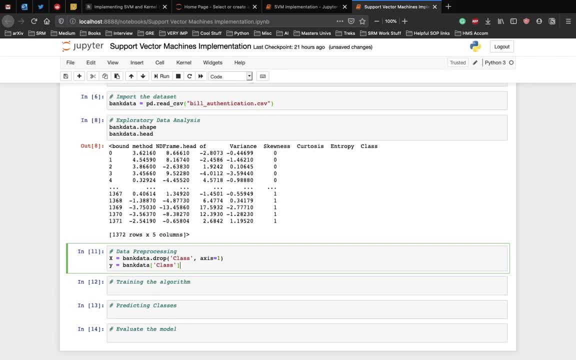 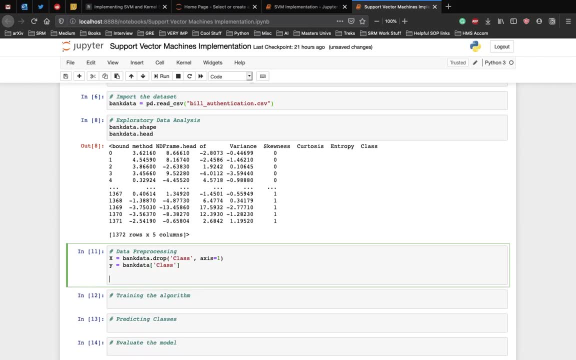 of time. x variable contains attributes, while y variable contains corresponding labels. Once the dataset is divided into attributes and labels, the final preprocessing step is to divide the data into training and test sets. Luckily, the model selection library of the cyclic learn library contains the train test split method that allows us to divide. 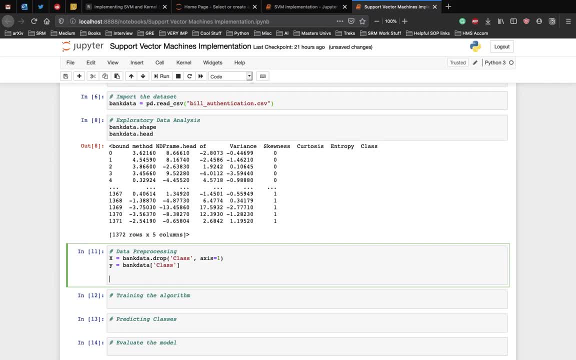 the data into training and test sets. to seamlessly divide the data into training and test sets, Let's write the code for that: xTrain, xTest, yTrain, yTest is equal to train test split x- y, and we want the test size to be 3%. 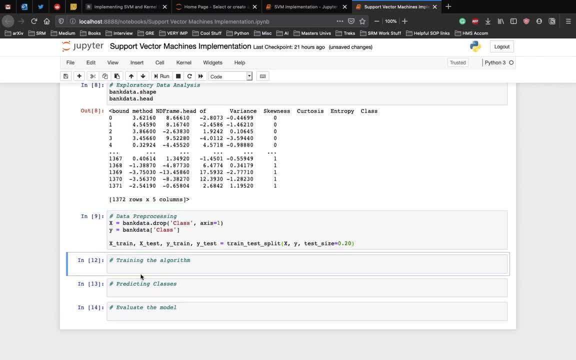 We have divided the data into training and testing sets. Now is the time to train our SVM on the training data. Scikit-learn contains the SVM library, which contains built-in classes for different SVM algorithms. Since we are going to perform a classification task, we will use the support vector classifier class, which is written as SVC in the Scikit-learn's SVM library. 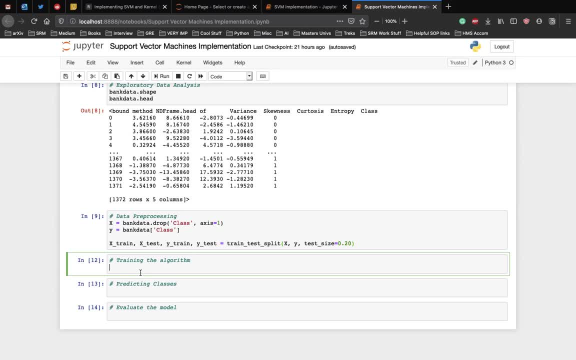 This class takes one parameter, which is the value of the class. This is the kernel type. This is very important. In the case of a simple SVM, we simply set this parameter as linear, since simple SVMs can only classify linearly separable data.